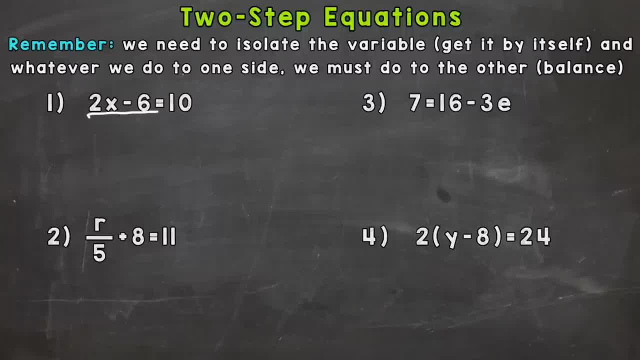 So how do we get rid of that 6 from the left side? Well, we can add 6.. That will cancel those 6s out or give us a 0.. So we can get rid of that 6 from the left side. So we can add 6.. That will cancel those 6s out or give us a 0. 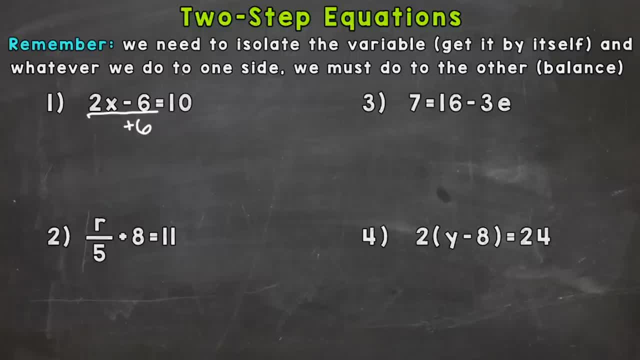 0. So remember, whatever we do to one side we have to do to the other. So if we add 6 to the left, we need to add 6 to the right. A negative 6 or minus 6 plus 6 gives us that 0, and 10 plus 6. 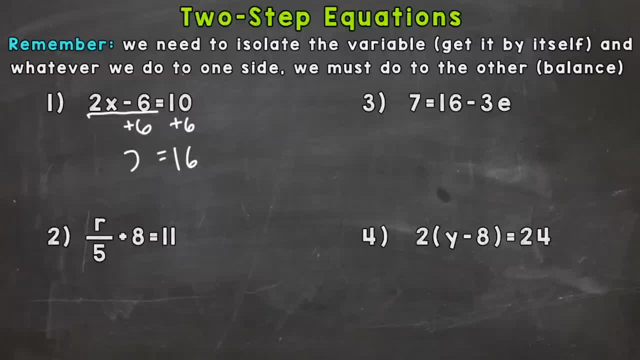 is 16.. So on the left side we're left with 2 times x or 2x. So we don't have the variable completely isolated yet, but we're almost there. So we have 2 times x. So how do we get rid of that? 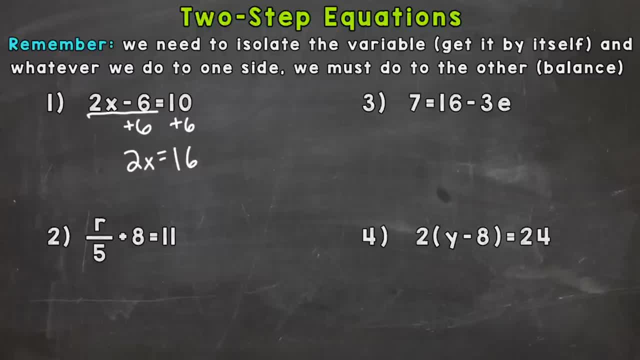 2?? We need to either make it a 0 or a 1.. So the opposite of multiplying by 2 would be dividing by 2.. That would give us 1x on that side, which is the same as just x. So let's divide both sides. 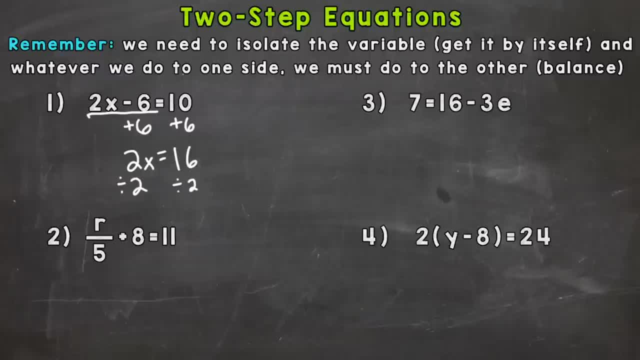 by 2, and that leaves us with x Equals. 16 divided by 2 is 8.. Now let's plug in that 8 into the original equation and see if we get the correct answer. So 2 times 8 minus 6 equals 10.. It's always a good idea to see if 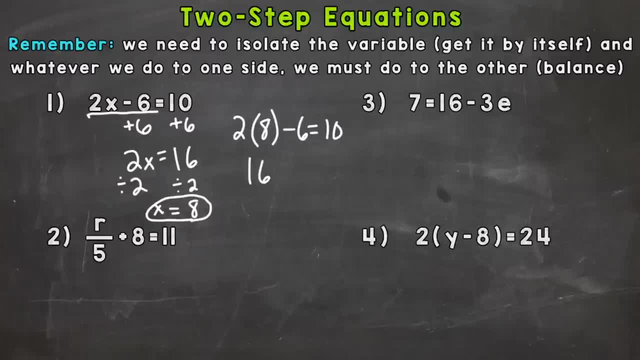 that answer works out: 2 times 8 is 16.. Minus 6 does give us that 10.. So we have the correct answer: x equals 8.. So for number 2, we have r divided by 5 plus 8 equals 11.. So we need to get that r by. 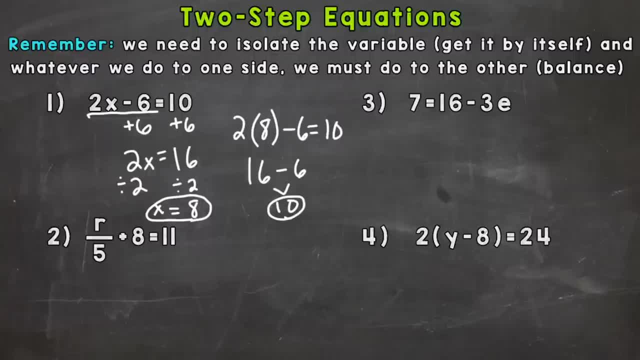 itself. So let's do the reverse order of operations to undo the left side of the equation. So let's get rid of that 8 first, So we have plus 8.. So the opposite: let's subtract 8 from both sides to begin to isolate the r. 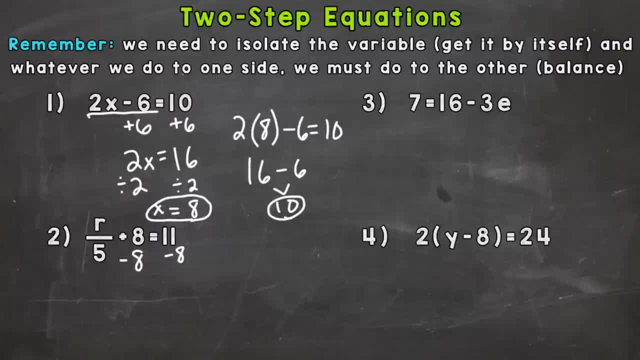 So a positive 8 and a negative 8 there minus 8, gives us 0. And 11 minus 8 gives us 3.. So on the left side we're left with r divided by 5.. So let's get rid of the 5 from the left side. What's the opposite of? 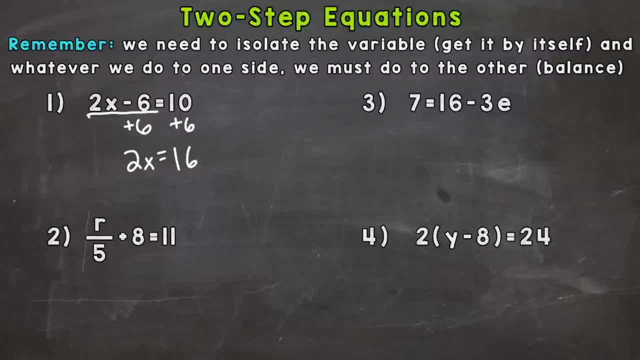 completely isolated yet, but we're almost there. So we have 2 times x. So how do we get rid of that 2?? We need to either make it a 0 or a 1.. So the opposite of multiplying by 2 would be dividing. 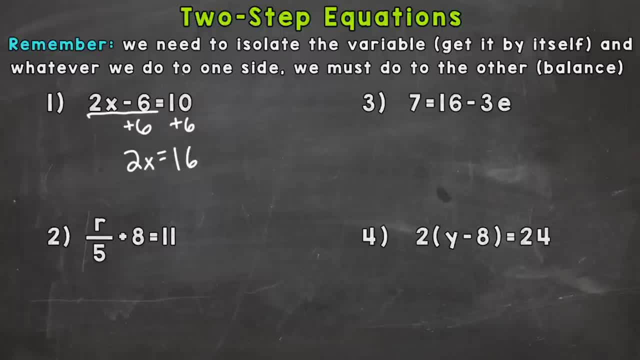 by 2.. That would give us 1x on that side, which is the same as just x. So let's divide both sides by 2, and that leaves us with x Equals 16 divided by 2 is 8.. Now let's plug in that 8 into the original equation and see if we 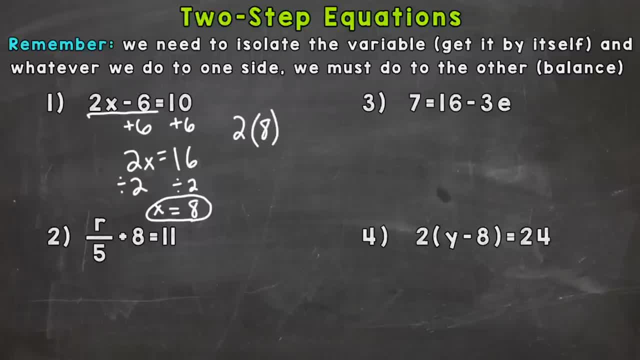 get the correct answer. So 2 times 8 minus 6 equals 10.. It's always a good idea to see if that answer works out. 2 times 8 is 16. Minus 6 does give us that 10.. So we have the correct. 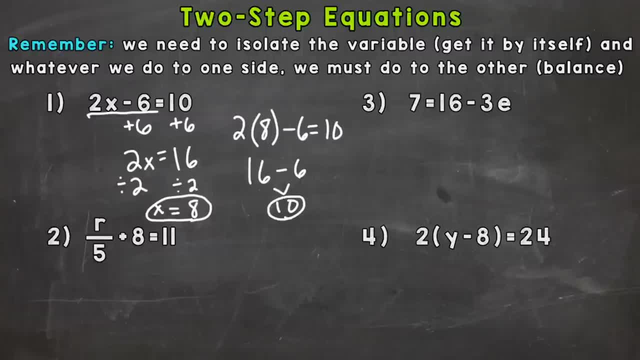 answer: x equals 8.. So for number 2, we have: r divided by 5 plus 8 equals 11.. So we need to get that r by itself. So let's do the reverse order of operations to undo the left side of the equation. So let's. 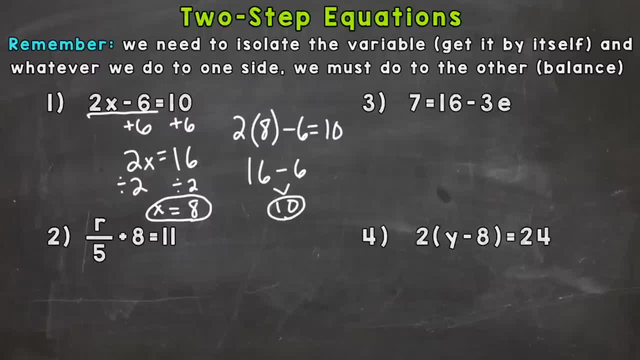 get rid of that 8 first, So we have plus 8.. So the opposite. let's subtract 8 from both sides to begin to isolate the r. So a positive 8 and a negative 8 there minus 8, gives us 0. And 11 minus 8 gives us 3.. So on the left side, 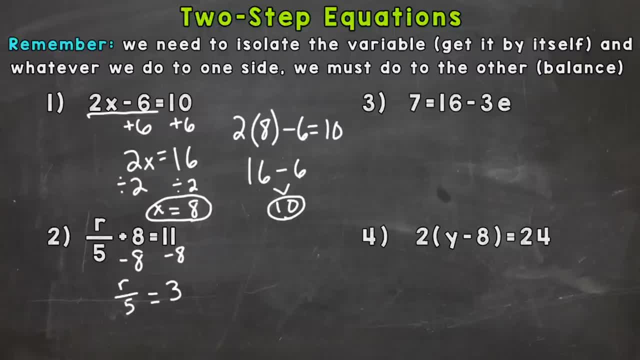 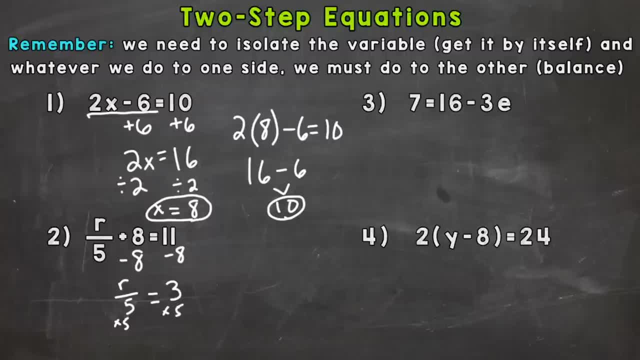 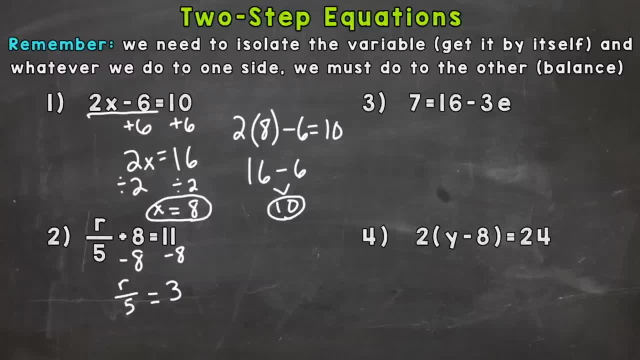 divided by 5?? Dividing by 5.. Well, multiplying by 5.. So let's multiply both sides by 5.. By 5. And we get r equals. well, 3 times 5 is 15.. We isolated the variable and it equals. 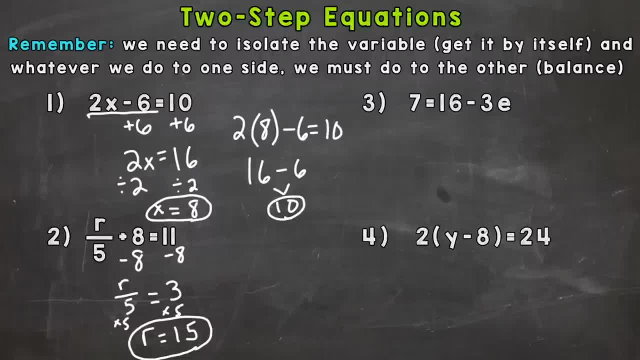 15.. So on the left-hand side I just want to mention we had r divided by 5,- that last step, And we times by 5, which would technically give us r over 1 or r divided by 1, which is just r. This is isolating the variable right here, if you get to multiplying that variable. 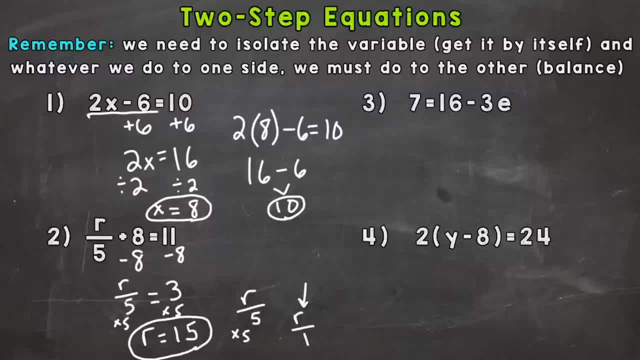 by 1 or dividing that variable by 1.. So let's plug in that 15 and see if we get the correct answer here. So I'm running out of room a little bit, I'll fit it in here. So 15 divided by 5 is: 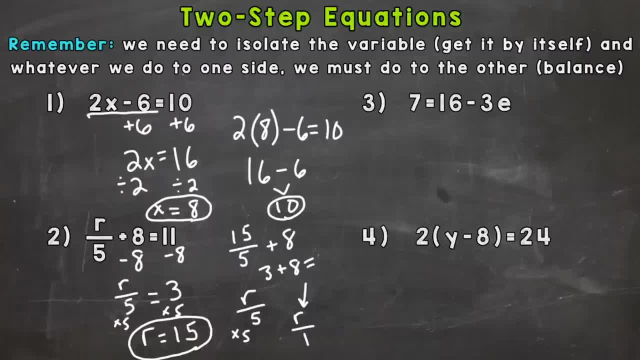 3. Bring down our 8 and we end up with 3 plus 8, which gives us the 11 we wanted. So let's go over to number 3 here, where we have 7 equals 16 minus 3e, So the equation looks a. 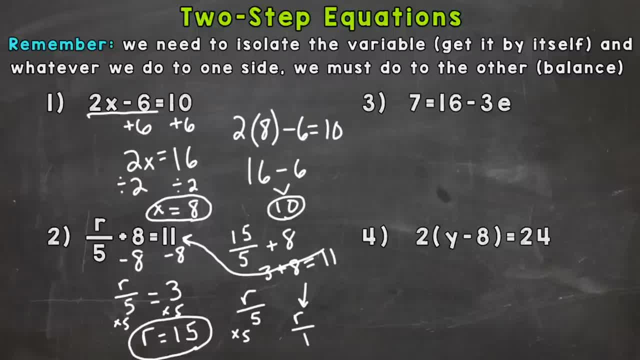 little different than numbers 1 and 2.. We have the variable on the right hand side, but it's the same exact thing that we did for numbers 1 and 2.. So we need to isolate that e So undo that right side of the problem. So let's get rid of the 16. 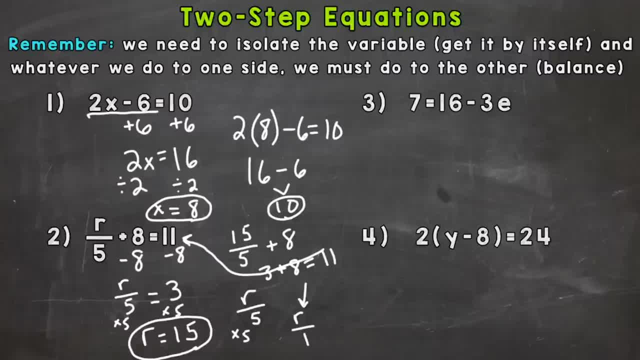 first. So we have a positive 16 on the right hand side. So the opposite would be subtracting 16. in order to get rid of it, Let's do minus 16 on the left hand side as well. So 16 minus 16 gives. 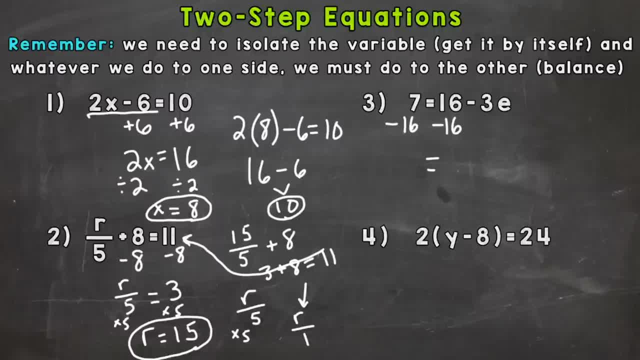 us that 0.. 7 minus 16 gives us that 0. So we have a positive 16 on the right hand side. So we need to do the opposite of multiplication in order to get the e by itself. So let's divide both sides. 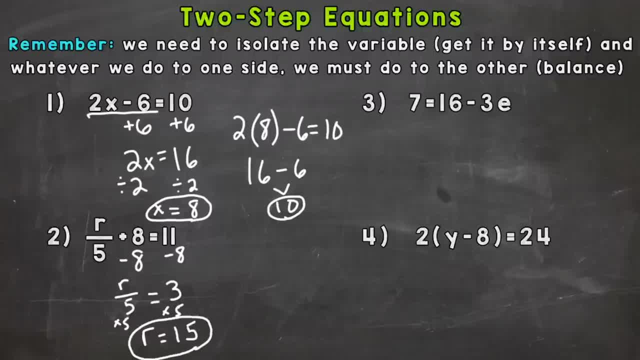 We isolated the variable And it equals 15.. So on the left-hand side, I just want to mention we had r divided by 5,- that last step- And we times by 5, which would technically give us r over 1, or r divided by 1.. 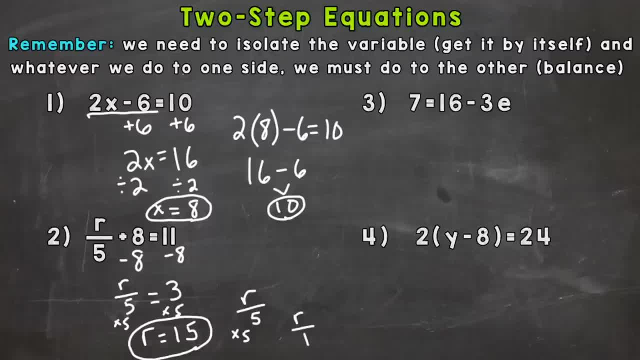 Which is just r. This is isolating the variable right here, if you get to multiplying that variable by 1, or dividing that variable by 1.. So let's plug in that 15 and see if we get the correct answer here. 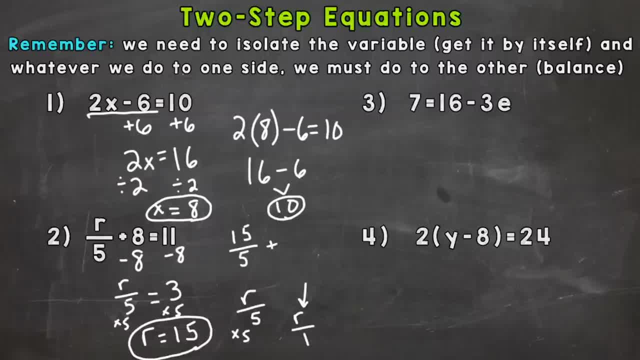 So I'm running out of room a little bit. I'll fit it in here. So 15 divided by 5 is 3.. Bring down our 8. And we end up with 3 plus 8. Which gives us the 11 we wanted. 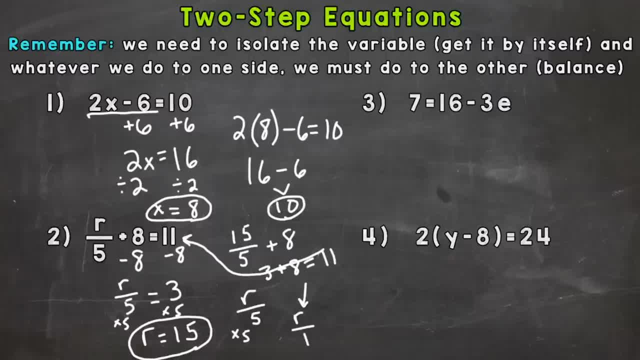 So let's go over to number 3 here, where we have 7 equals 16 minus 3e, So the equation looks a little different than numbers 1 and 2.. We have the variable on the right-hand side, But it's the same exact thing that we did for numbers 1 and 2.. 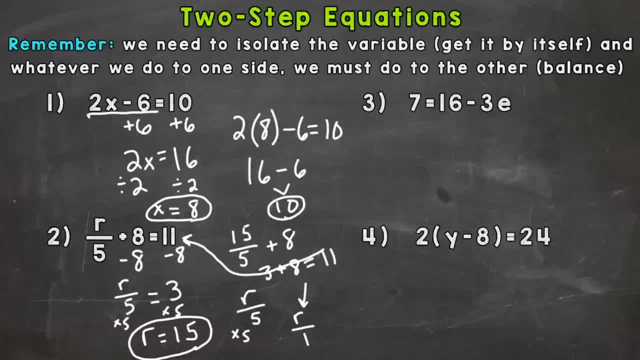 So we need to isolate that e So undo that right side of the problem. So let's get rid of the 16 first. So we have a positive 16 on the right-hand side. So the opposite would be subtracting 16 in order to get rid of it. 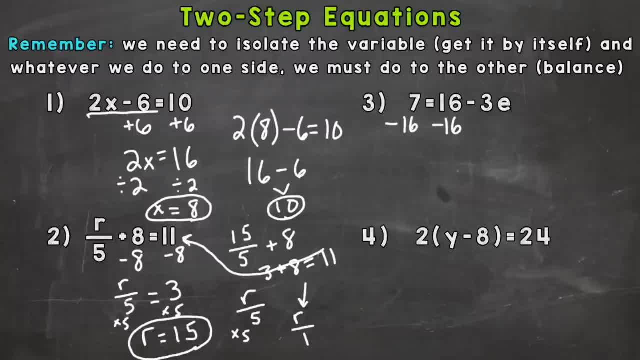 Let's do minus 16 on the left-hand side as well. So 16 minus 16 gives us that 0.. 7 minus 16 gives us a negative 9.. We're left with Negative 3e on the right side. 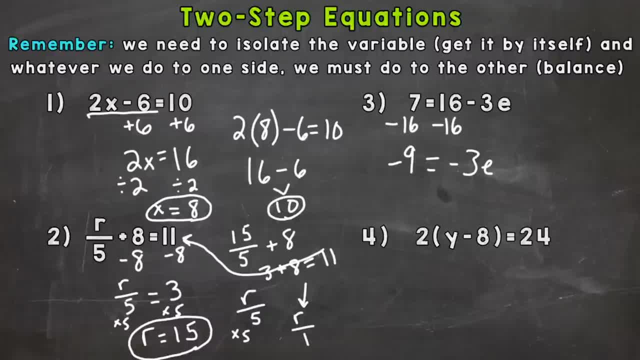 So that's multiplication. So we need to do the opposite of multiplication in order to get the e by itself. So let's divide both sides by negative 3.. Negative 9 divided by negative 3 gives us a positive 3. And we're left with e over 1, which is the same thing as just e. 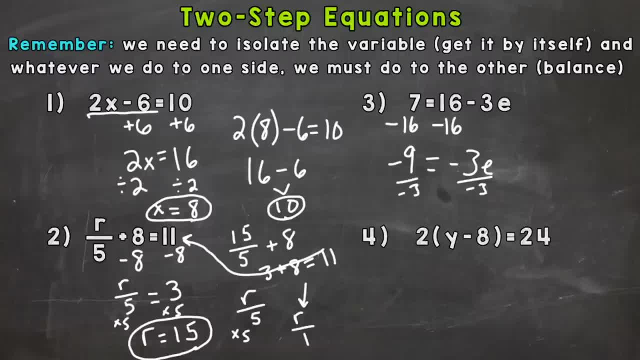 by negative 3.. Negative 9 divided by negative 3 gives us a positive 3. And we're left with e over 1, which is the same thing as just e. We isolated the variable, So e equals 3.. Let's plug it back in and see if that works. 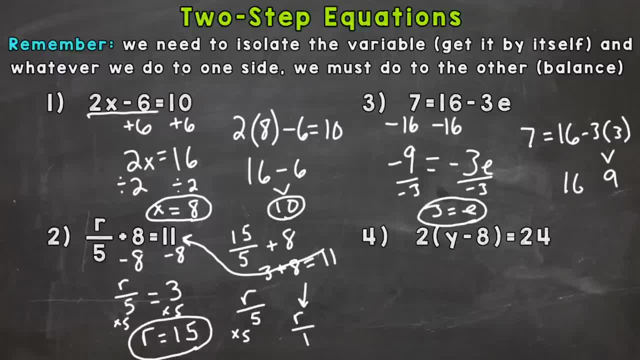 3 times 3 is 9.. Bring down our 16.. 16 minus 9 does give us that 7 that we were looking for on the left hand side of that equation. So we were correct: e equals 3.. And lastly, number 4.. So we have some. 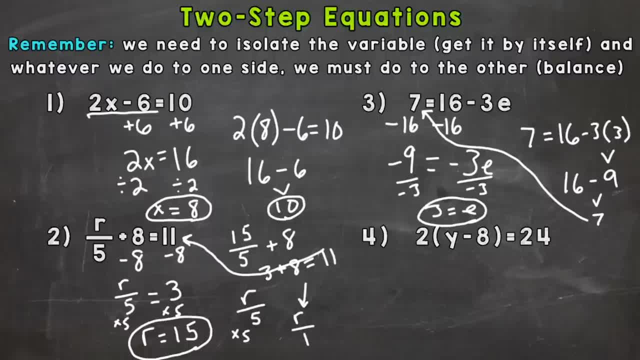 parentheses in this one And we need to get y by itself or isolate the variable y. So we have 2 times parentheses, y minus 8 and parentheses equals 24.. So we need to do the opposite. Remember, we need to undo that side, the left hand side of the equation. 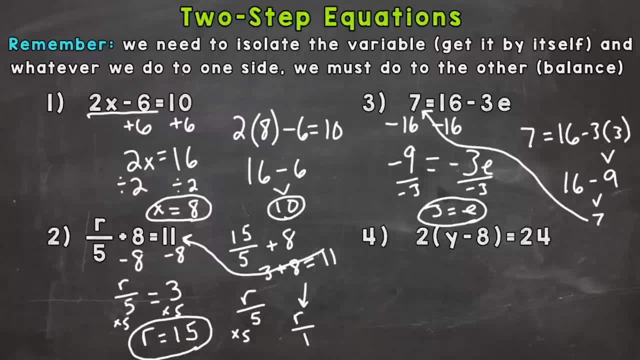 And we're going to actually divide both sides by 2 to undo that 2 that is outside of the parentheses. So 2 divided by 2 is 1.. That gives us 1 outside of the parentheses there, which is just going to leave us with y minus 8, because anything times 1 is just that number or expression itself. So we 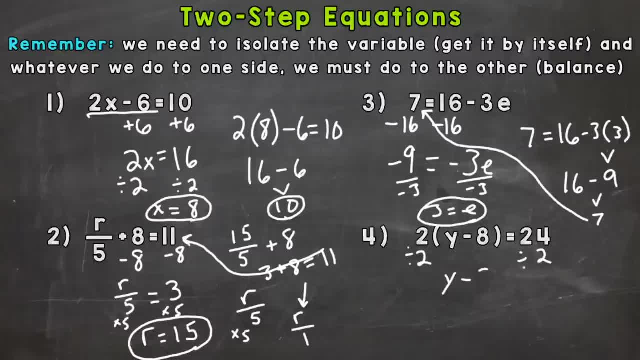 just have y minus 8. And we're going to divide both sides by 2 to undo that 2, that is outside of the parentheses, and then 24 divided by 2 is 12.. So now we have y minus 8 equals 12.. So we need to get rid of that. 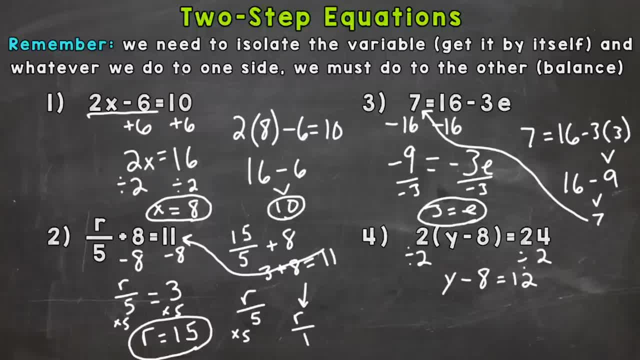 minus 8.. Undo that part of the left hand side of the equation in order to isolate the y. So we need to add 8 to both sides in order to isolate the y. So a minus 8 and a plus 8 gives us a 0. Those 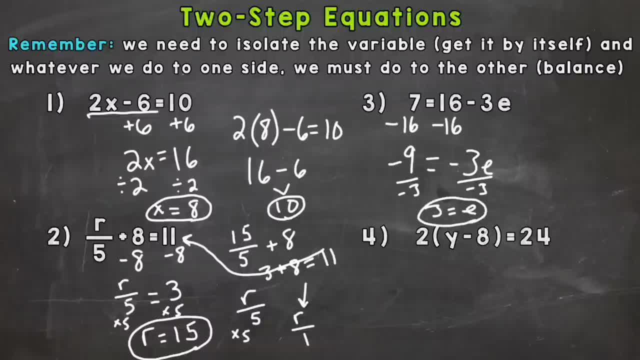 We isolated the variable, So e equals 3.. Let's plug it back in and see if that works. 3 times 3 is 9.. Bring down our 16.. 16 minus 9 does give us that 7 that we were looking for on the left-hand side of that. 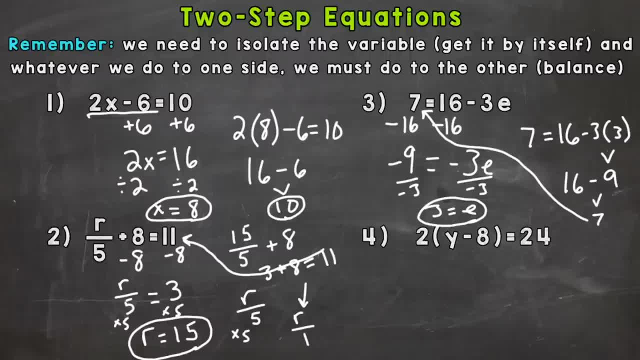 equation. So we were correct: e equals 3.. And lastly, number 4. So we have some parentheses in this one and we need to get y by itself or isolate the variable y. So we have 2 times parentheses: y minus 8, end parentheses, equals 24.. 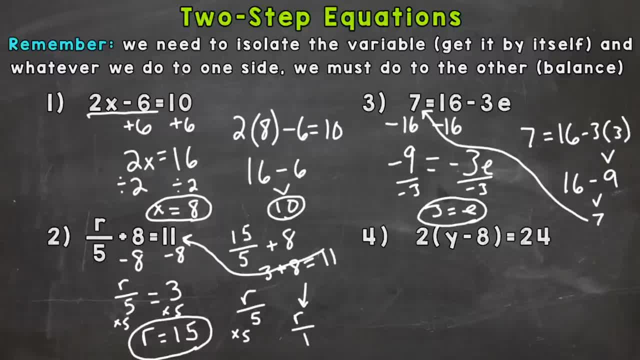 So we need to do the opposite. Remember, we need to undo that side, the left-hand side of the equation, and we're going to actually divide both sides by 2.. 2 divided by negative 3. We'll never be able to undo that 2. that is outside of the parentheses. 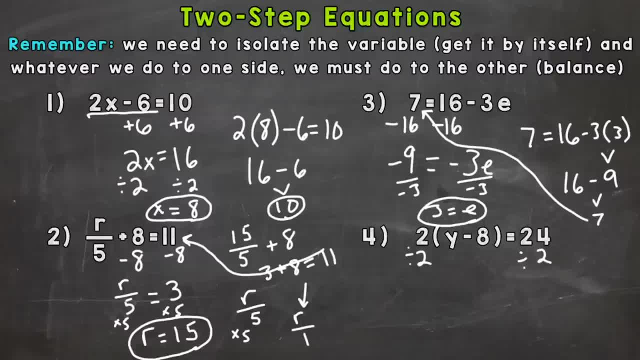 So 2 divided by 2 is 1.. That gives us 1 outside of the parentheses there, which is just going to leave us with y minus 8, because anything times 1 is just that number or expression itself. So we just have y minus 8.. 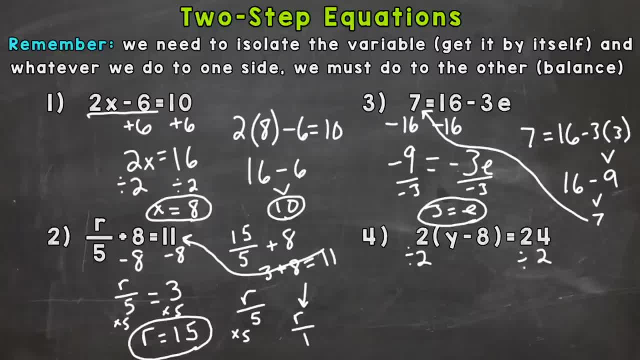 And then 24 divided by 2 is 1.. So if I just have that y minus 8. Why would I forget that? Why would I forget that? Yeah, Yeah, Yeah, Yeah, Yeah by 2 is 12.. So now we have y minus 8 equals 12.. So we need to get rid of that minus 8.. Undo that, 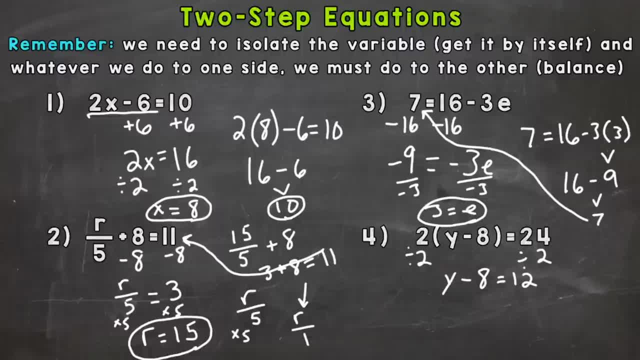 part of the left hand side of the equation in order to isolate the y. So we need to add 8 to both sides in order to isolate the y, So a minus 8 and a plus 8 gives us a 0. Those cancel out. 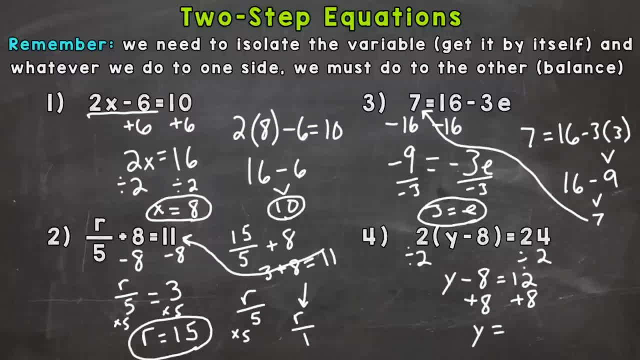 So we're left with y, and 12 plus 8 gives us 20.. So y equals 20.. Let's plug it back into the equation to see if this gives us the answer 24 that we're looking for. 20 minus 8 is 12.. Bring down the 2.